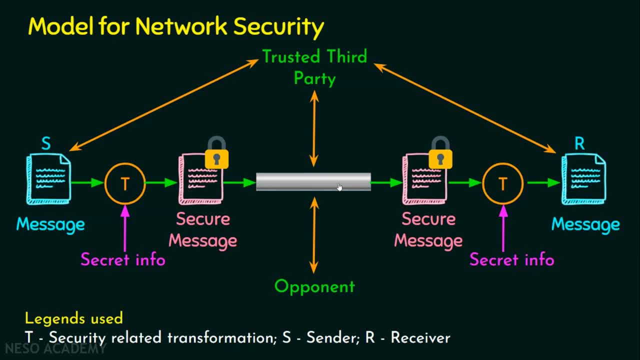 Now this secure message can travel on the internet and it will definitely reach the destination. Now, when the destination, that is, the receiver, receives the message, he will receive only the ciphertext. that is the secure message. What the receiver has to do: The receiver: after receiving the ciphertext or the secure message, it should be converted. 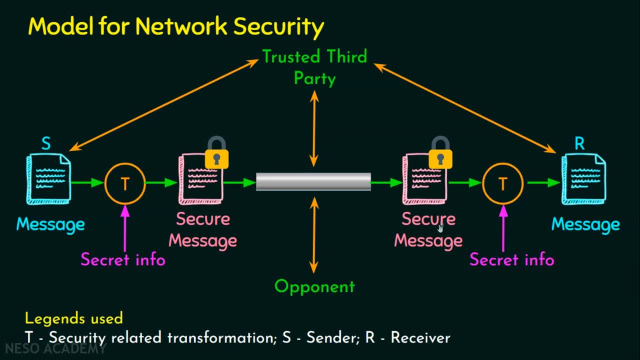 back to its plaintext form. So the receiver will be decrypting the message. So again, a security related transformation is applied, taking the ciphertext as an input and secret information as another input. Now this transformation in the receiver side can be a decryption algorithm and this decryption 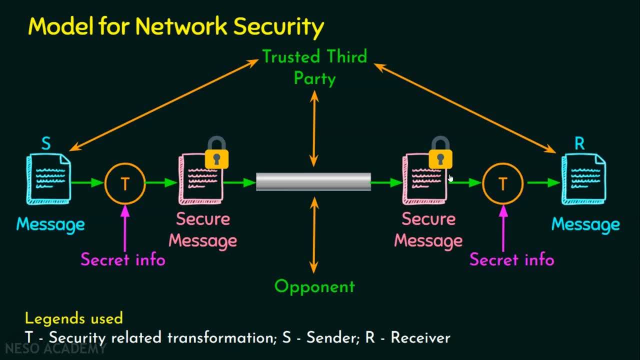 algorithm will convert the ciphertext or the secure message back to the original message, which is the plaintext. Now this is done at the receiver side, So simply, sender creates the message, gives that message to the transformation function or an encryption algorithm. With the help of the key, this plaintext is converted into ciphertext which is referred. 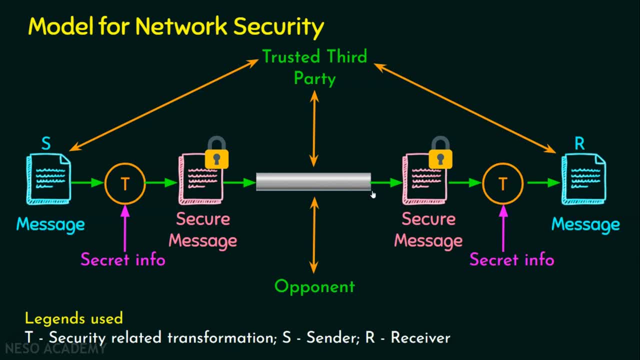 as a secure message and this secure message can travel on the internet and this secure message will be received by the receiver and receiver will decrypt this message. and this security related transformation will take the secure message as an input and it will also use a secret information which can be a key, and it gives the plaintext back. 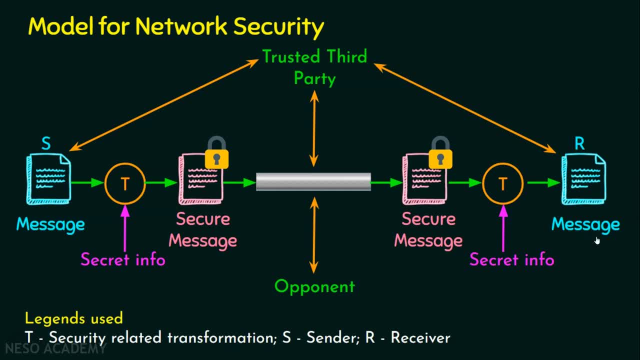 This is the message. Now, in this whole scenario, we can notice that there is a security related transformation Which is in both sender side as well as in the receiver side. We know S is the sender, R is the receiver, So sender and receiver are not communicating messages, but they are communicating secure. 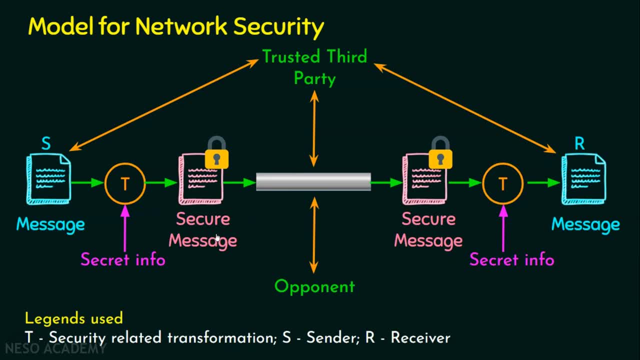 messages. So this is what the ultimate intention of a network level security model is. Now, in this scenario, there are certain situations where sender and receiver must use a third party service, Say, if there is a sender and the receiver is going to be a web server. 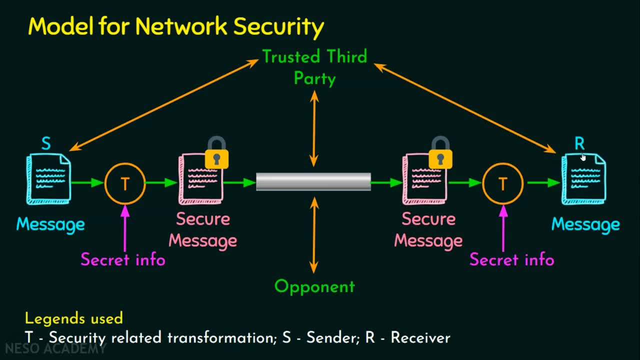 For example, say: if you want to access googlecom, Now sender wants to access actually googlecom. In that case, sender and receiver are obviously going to exchange secure communication only. We can also take one more example: a banking server, Since banking server deals with confidential information, so sender and receiver are again. 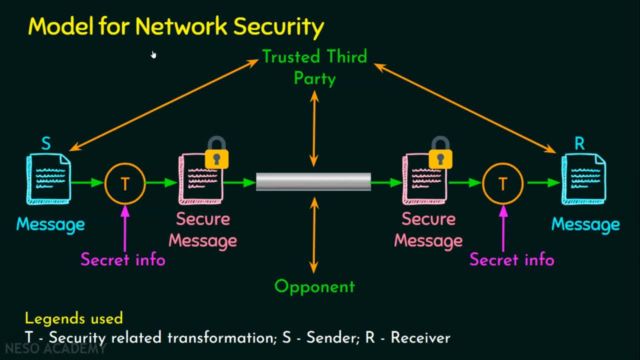 going to communicate using this secure message concept or the network security model. Let's assume that we are going to access the banking server or google server, whatever we want. Let's assume it is a server which uses SSL certificates. Now this SSL certificates will be provided by a trusted third party. 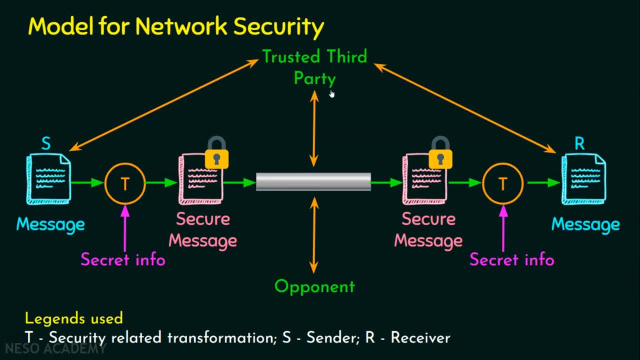 We will see about the role of trusted third party in the last chapter of this subject. For time being, just understand. a trusted third party is involved between the sender and the receiver in order to handle certain level of security functions. Also, you can see here there is an opponent or attackers who will be at this level. 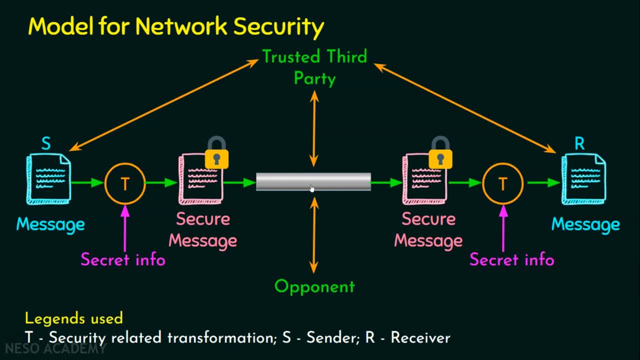 Why they will be at this level? Because they will be obviously on the internet. They will be sniffing the conversation or they will be trying to know what is the data that is being exchanged between the sender and the receiver. So they will be normally getting the ciphertext and that's why opponent is placed here. 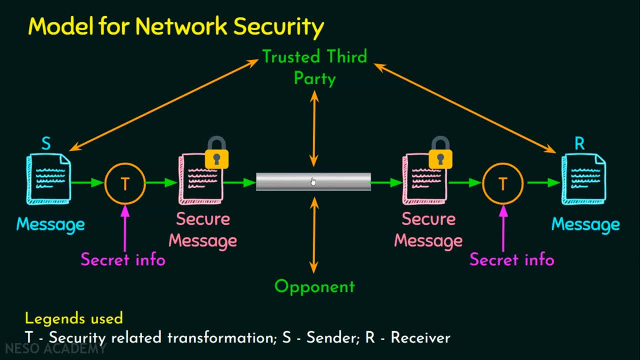 So they will get secure messages only. But the real security lies with the encryption algorithm, which uses a very strong key. If it is a very simple algorithm and the key is a very smaller one, then obviously attacker can easily break that. So the security is actually relying with this encryption algorithm and the secret information. 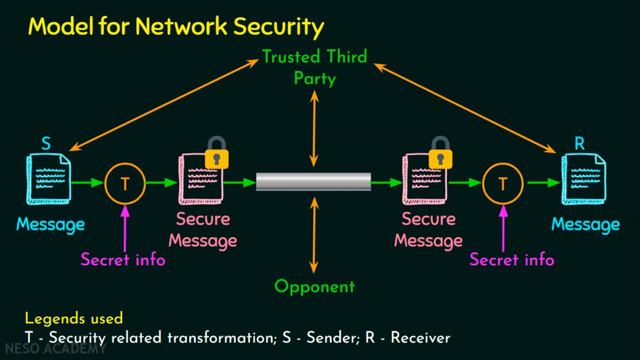 which is a key which should be of large number of bits. You might have one question in your mind: Why am I referring the encryption algorithm as a security level transformation T? Why don't I directly use it as E for encryption? We are dealing with the model for network security, where encryption is one of the ways. 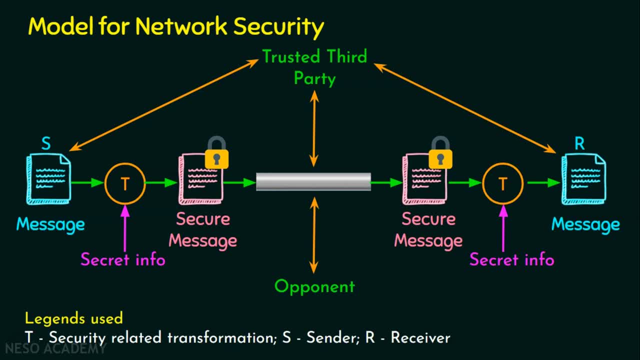 to provide security. It can be steganography also, Where in steganography we are going to hide the data inside the network In some other form. we are going to talk about that in the upcoming lecture anyway, But we need to understand that we are not going to send messages. 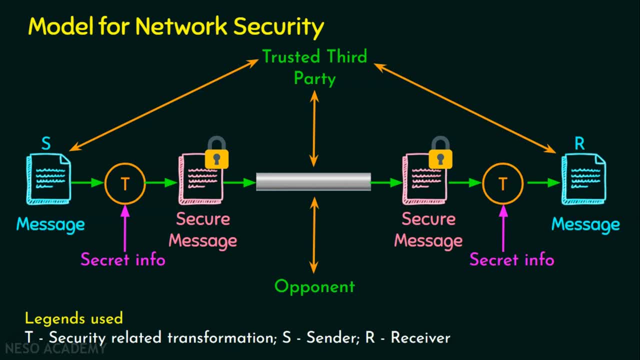 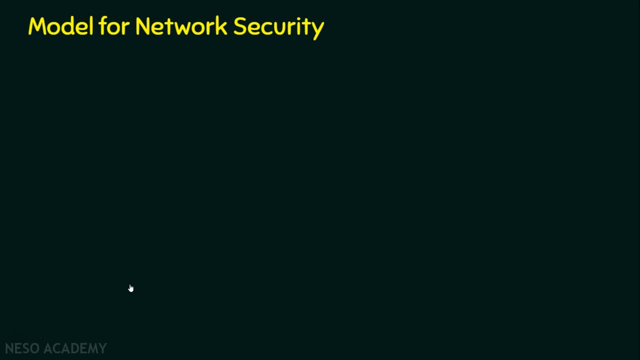 Rather, we are going to send secure messages over the internet so that no one can understand except the authorized parties. We are done with the model for network security. Let's now see the basic or major four tasks for designing the network security model. Basically, there are four tasks, as mentioned. 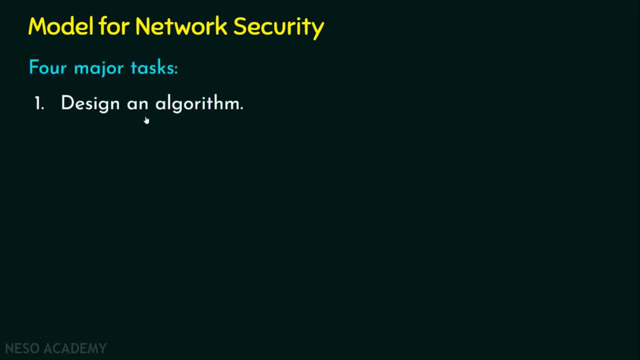 Number one is design an algorithm. So when we want to have a strong security feature, as I mentioned in the last slide that the real security relies on the encryption algorithm, This encryption algorithm is at the sender side and the decryption algorithm will be at the receiver side. 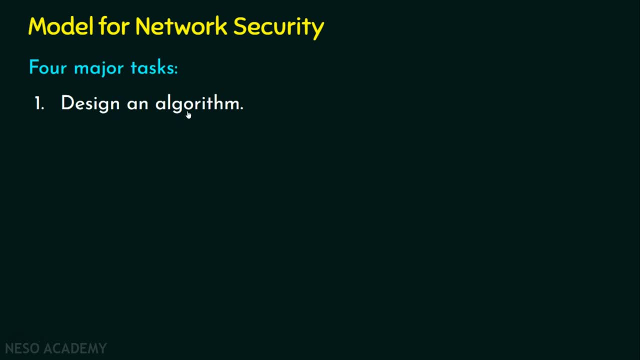 So we need to focus on designing a strong algorithm, which is considered to be the first major task. Let's now see the second major task: Generate the secret information. Let's take the encryption algorithm. The encryption algorithm is going to take two important inputs. 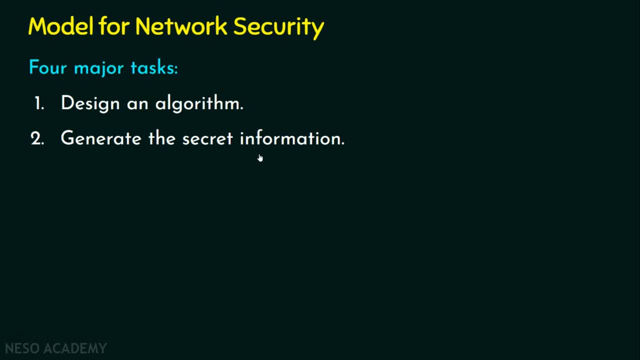 Number one is the plaintext and the second one is the key or some secret information. So the real security is relying on the secret information as well. If the key size is large enough, then the security is very high. So we need to focus on generating the secret information, which is of large number of bits. 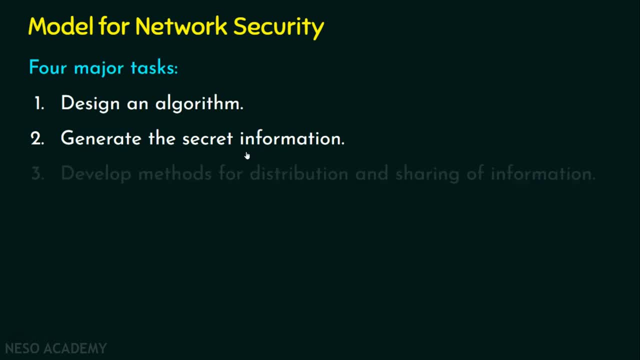 We are done with the second major task. Let's now move on to the third major task: Develop methods for distribution and sharing of information, because sender and receiver are going to use some keys right. Suppose, if the sender and receiver are going to use symmetric encryption, that is the 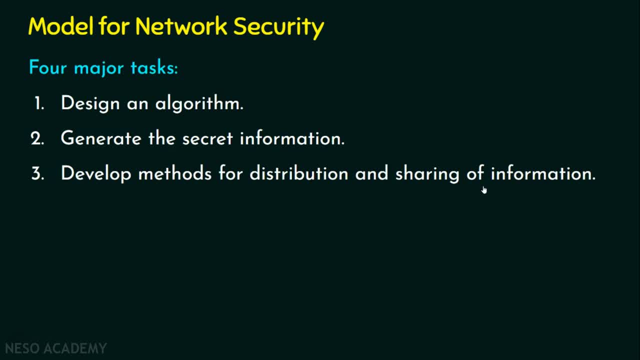 same key is used for encryption and decryption. Don't worry about the symmetric encryption or symmetric cryptography. We are going to see that in the upcoming lectures anyway, But for time being I am telling you, suppose, if sender and receiver are going to use symmetric 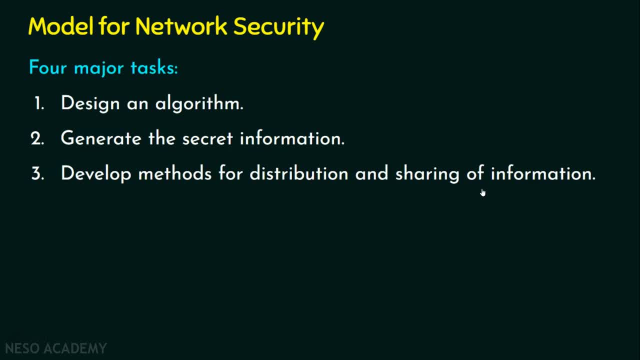 cryptography. it means same key is used for encryption and decryption, So in that case we need to focus on how this key is distributed. If the key is distributed on the internet and the sender and receiver are going to use it again, there are chances for the attackers to steal the key right. 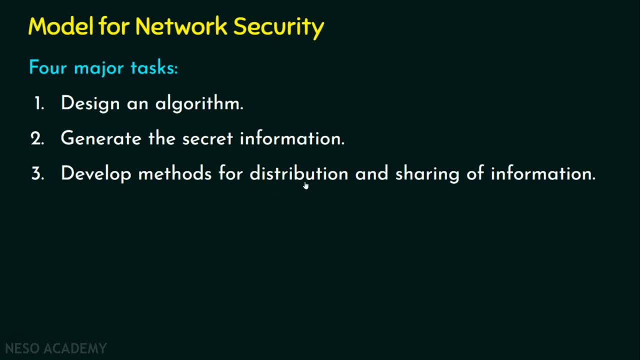 So we need to focus on some methods, or develop some methods, for distribution and sharing of some information. This information includes keys as well. Let's now move on to the fourth task: Specify a protocol, because this is very, very important. This security protocol only is going to be used by both sender and the receiver as well. 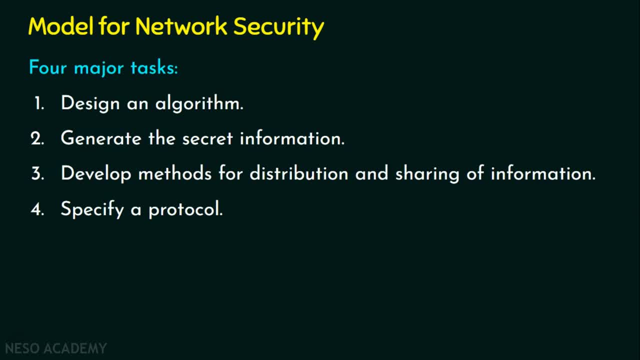 as on the internet, And the protocol will have a complete suite of all the required security essentials to the package So we can directly use it For the protocol. obviously sender and the receiver will be abiding by the rules and regulations offered by the protocol and obviously there will be security. 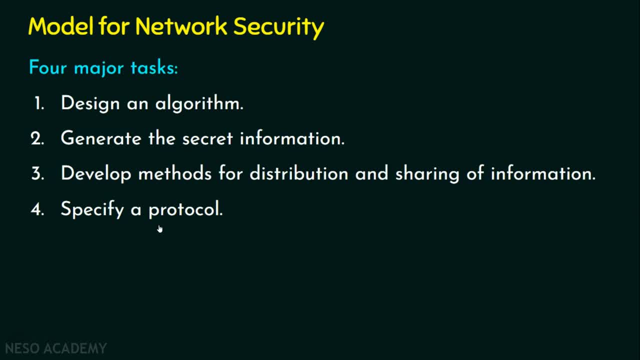 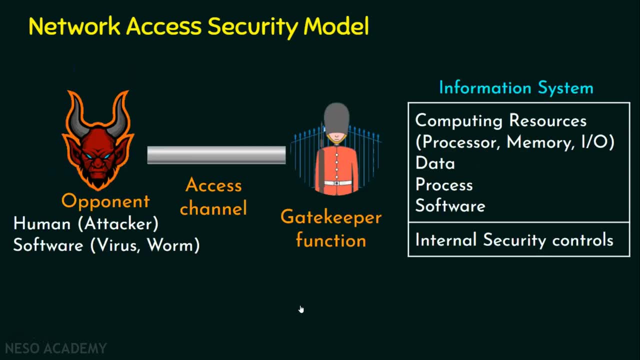 So these are the four major tasks that should be considered when we design a network security model. Before we conclude, let's see the model for network access security. Here is the model for network access security where you can find that there is an opponent. 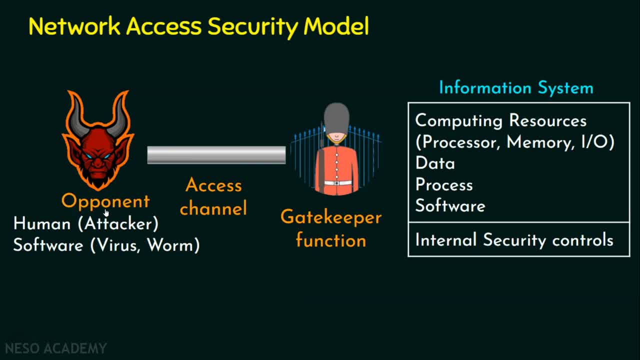 and this opponent we will normally call as an attacker. But please note, the opponent can be an attacker which is considered to be an human, or an attacker can be a software. This software may be a virus, worm, trojan or many malicious software are there. 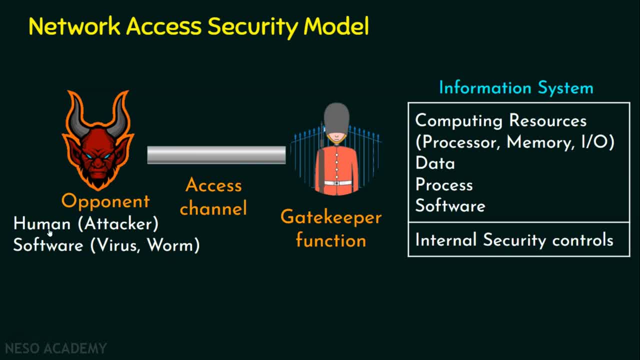 So simply opponent means it can be either a human or an automated program, which is the software. Obviously, we have our information system, which is considered to be a system which requires high degree of security. Now, what will be there in an information system? 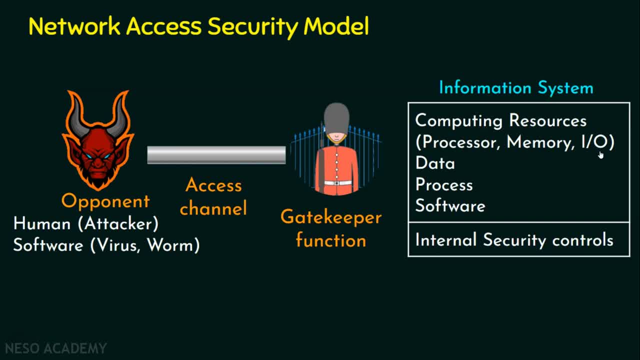 All the computing resources, like the processors, memory, IO, and this information system is going to have the main entity, the data. It will also have the process, It will also have software, Since all these important and vital elements are there in an information system. obviously. 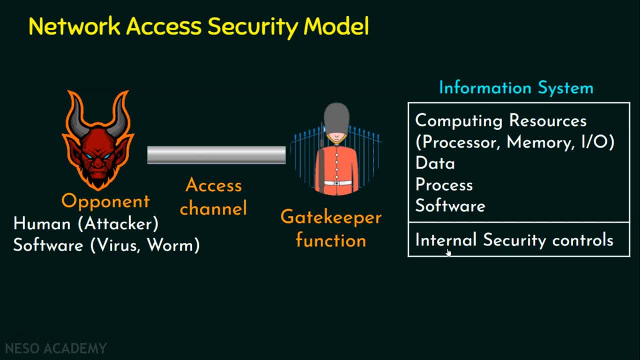 there will be some security levels. in the internal level, That is, in the information system, we will have internal security controls. These internal security controls will protect this information security to some extent, internally as well as externally, But the opponent will always try to intrude. 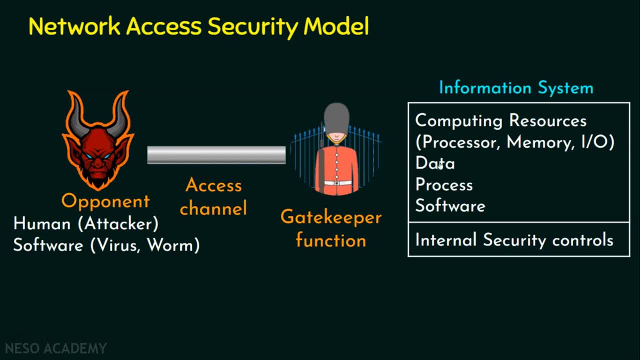 Let's try to intrude or gain access to this information system. In order to stop that, we need to have a gatekeeper function. Generally, this gatekeeper function can be a firewall or any security mechanism which filters the traffic before giving the data to the information system. 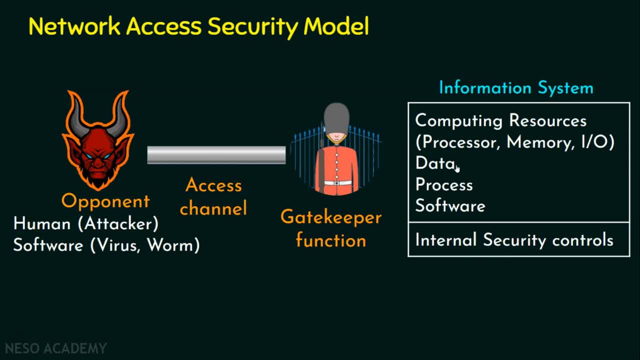 This internal security controls. example, antivirus programs will be there in the information systems or in all the systems inside the organization and this gatekeeper function will be filtering the traffic. So this gatekeeper function will filter If a legitimate user is accessing or an attacker is trying to intrude the network. so obviously, 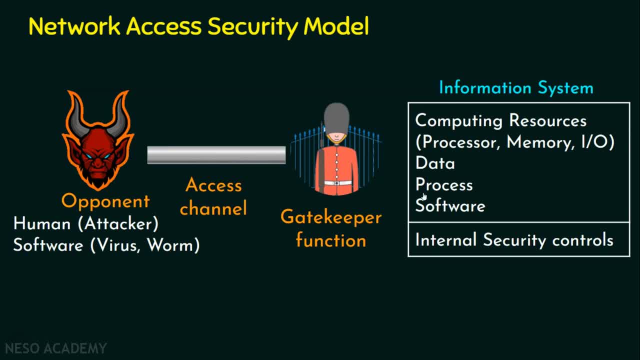 this access channel will be the internet. in order to do all this stuff, All the traffic that goes to the information system or comes out of the information system should go through the gatekeeper function. This gatekeeper function will analyze all the data traffic and it will say whether the traffic 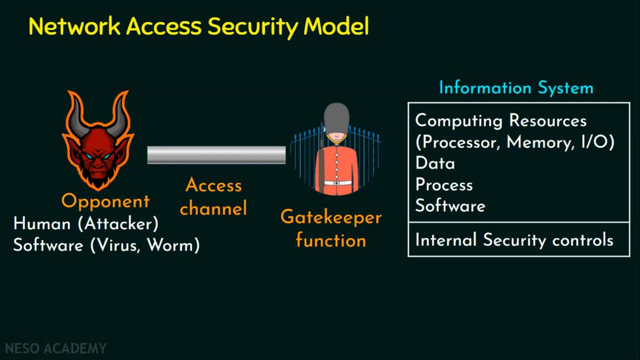 is permitted or not, And this is very essential because this gatekeeper function should be a very strong and a very diligent one. It can identify whether a legitimate user is accessing or sending the traffic, or a virus is attacking, or a human or an attacker is attacking.